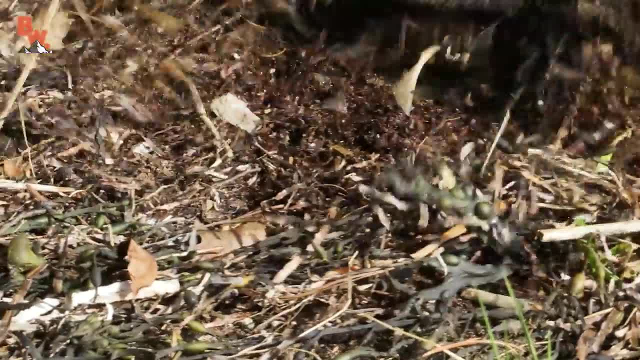 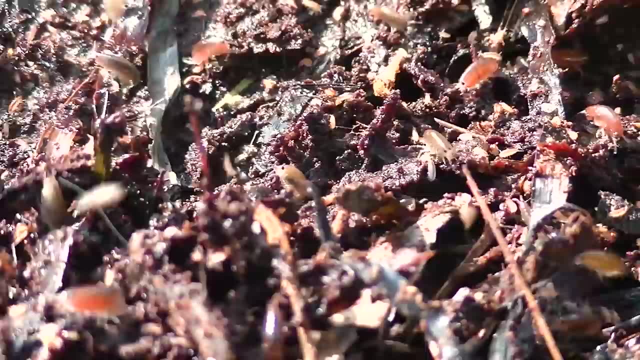 Watch Ready. Yeah, One, two. Oh my gosh, What Look at that? What Put my hand in there? Yeah, All right. All right Here, let me peel back some more. Oh jeez. 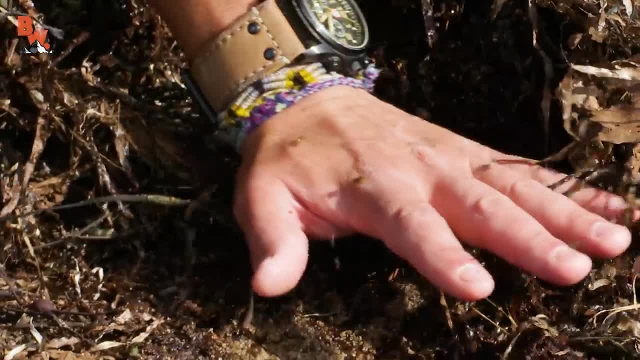 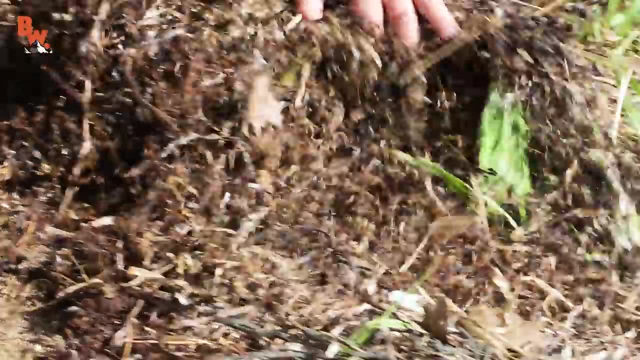 What's that? like? That feels really weird, but they're not biting me, They're just jumping on me Here. let me peel back this a little bit more. Look at that. There are like millions of them. Oh my gosh, That is crazy. 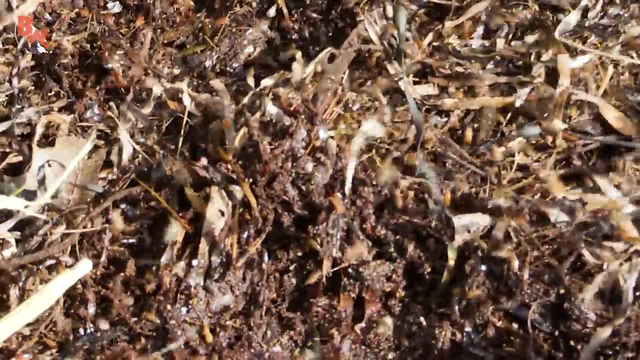 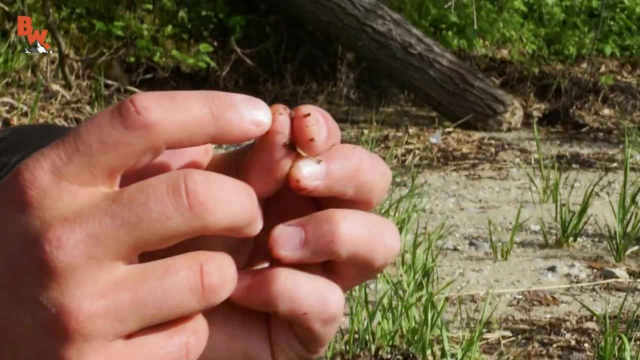 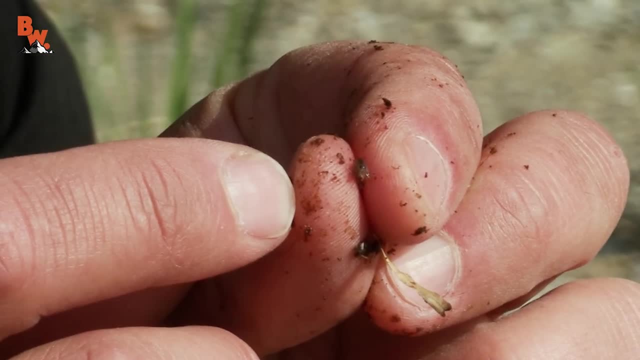 Whoa Got one. Yeah, Look, look, look, Right there. Can you see his little head sticking out? I believe that's a sand flea. Whoa, That is creepy. All right, Note to self: Don't lay on this beach. 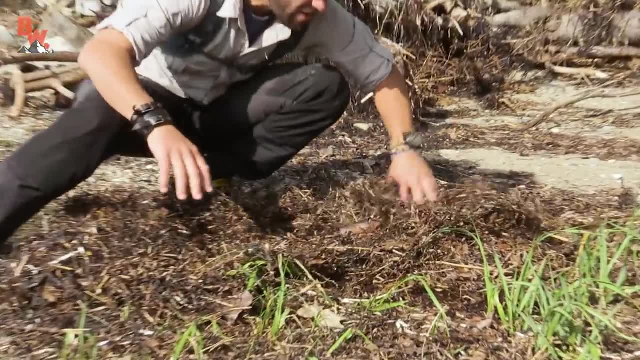 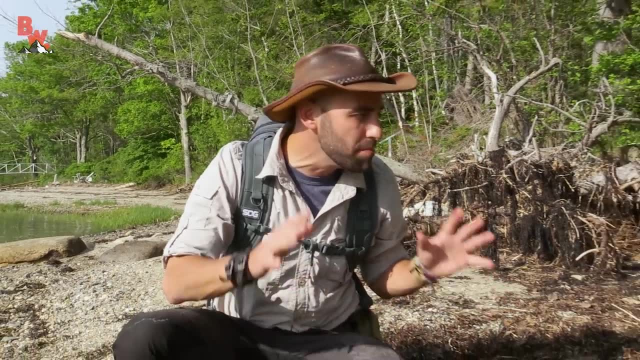 I'm just going to disperse some of this dead seaweed back out and cover up the sand flea city. I have never seen anything like that: Millions upon millions of sand fleas. All right, Let's head this way down the coastline and see what else we can find. 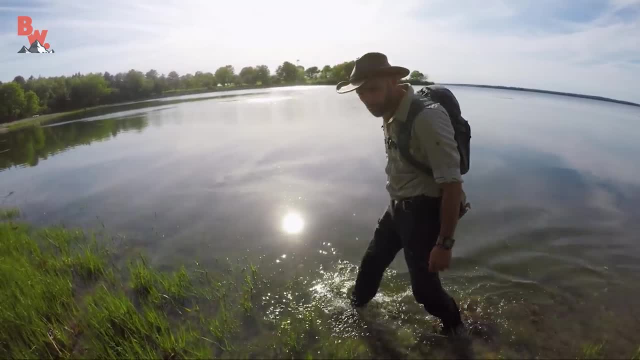 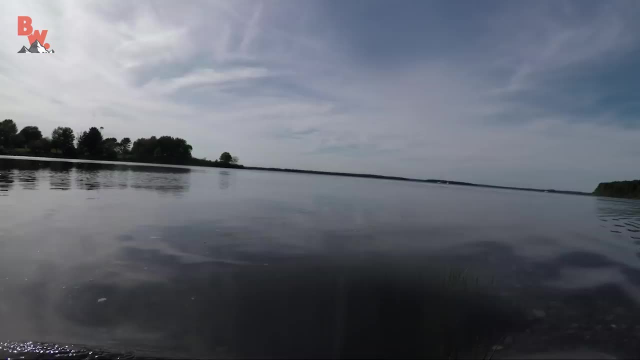 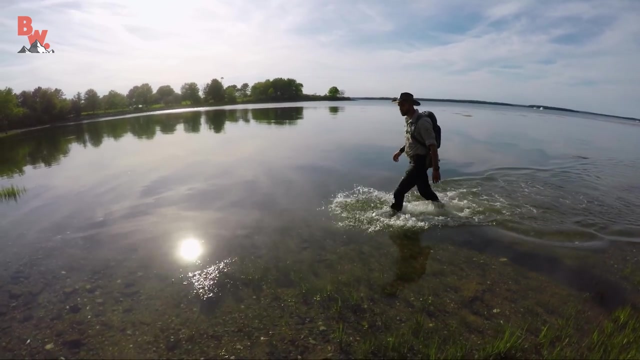 As we continue down the coastline, we soon realized it was unlike any low tide scenario we had explored before. I carefully examined potential hiding spots where animals may be waiting for the tide to return, But so far, aside from thousands of fleas, I wasn't seeing a single living creature. 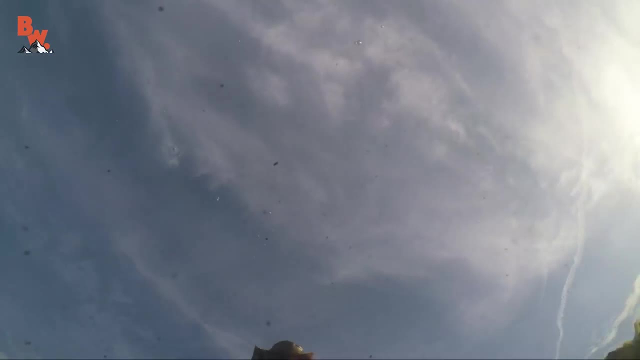 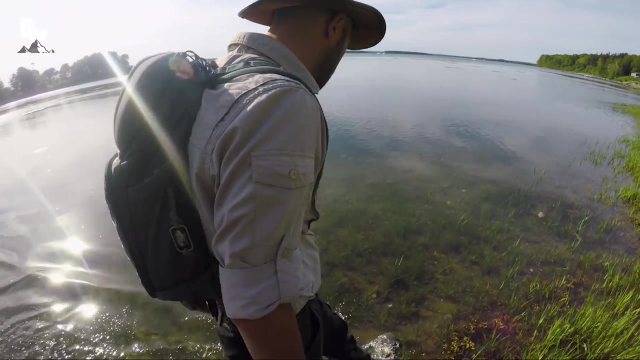 The sun was getting low in the sky when, all of a sudden, our luck took the perfect turn and put us right in the midst of an animal. we had always hoped to get up close for the cameras. We finally found a turtle. Oh, it's a turtle. 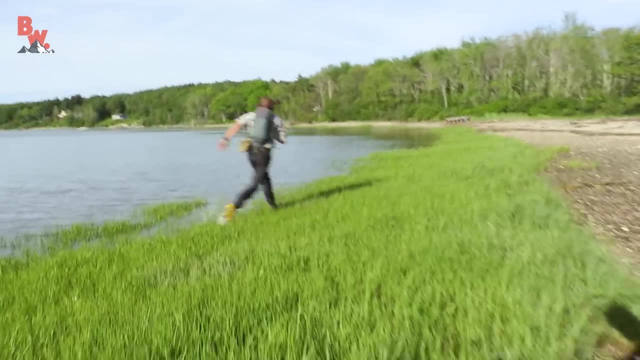 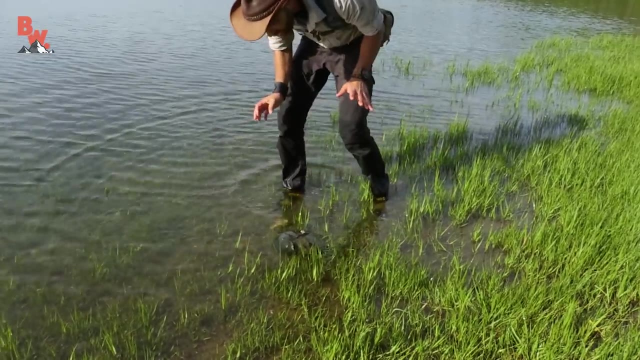 Oh, that's a horseshoe crab. What? Look at this. Is it alive? Oh, it is alive. Look at that. Yes, Wow, I thought that was a turtle. Oh my gosh, I just saw the lump. 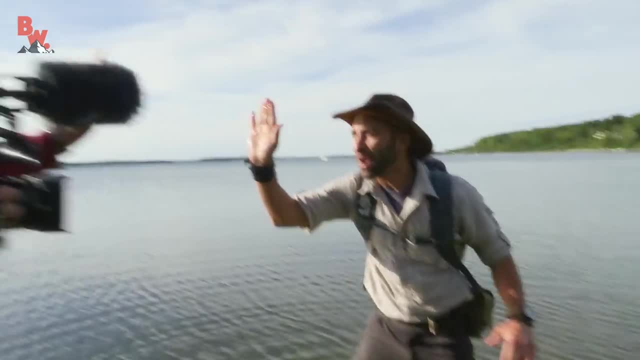 I thought it was a carapace. All right, Let's do this. I'm going to gently lift it up out of the grasses here. Let's see, Oh, it's strong. Look at that. Wow, Look at its tail going. 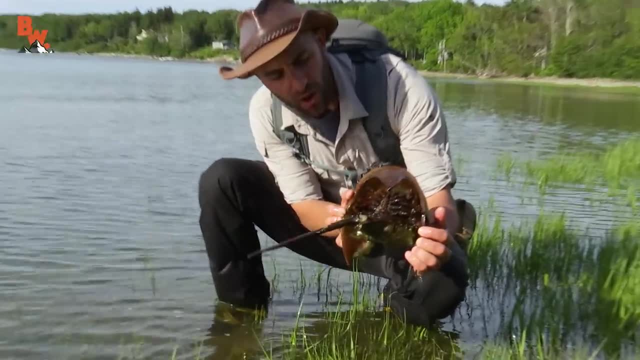 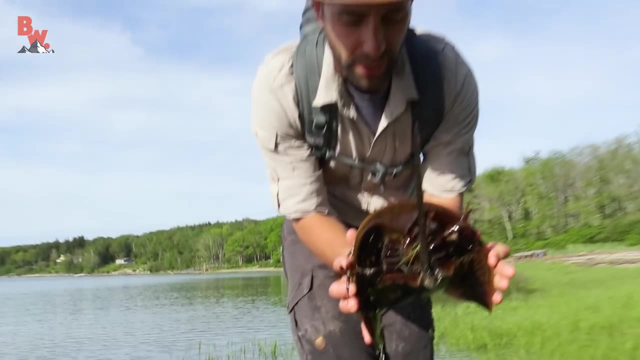 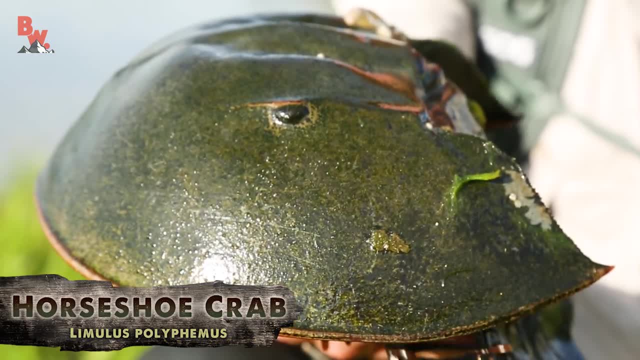 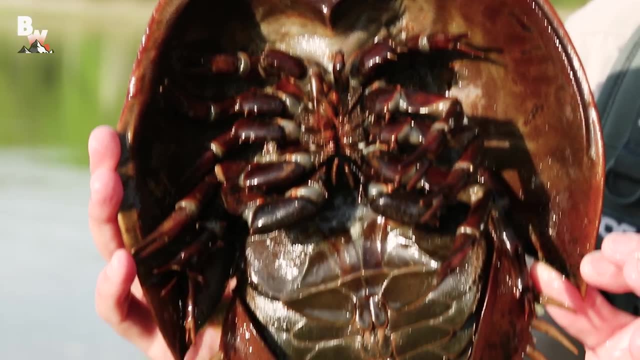 What a bizarre looking creature. Now you may be thinking, Coyote, is that thing going to pinch and bite you like crazy. No, They actually just have a little tiny mouth right in the center, and they have no stinger, no fangs, no teeth. 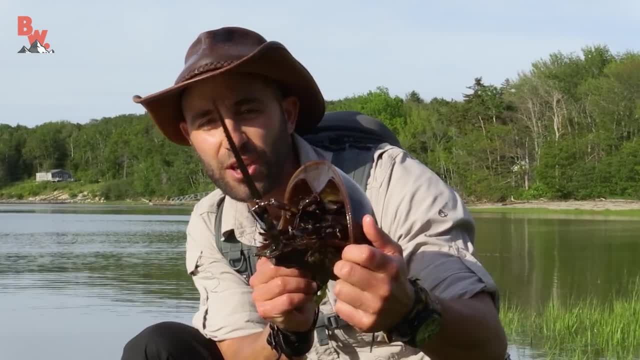 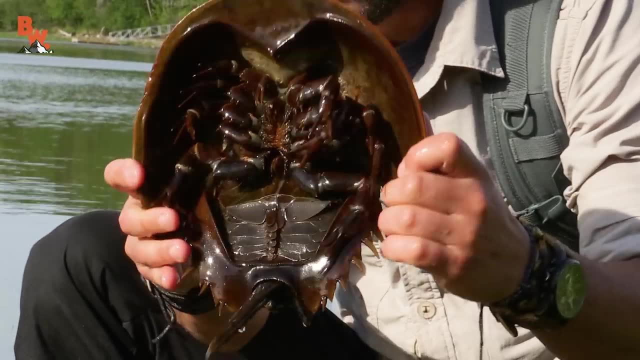 Look at that back tail. there They've gotten a bad reputation because of this tail. People think that that's venomous. It actually is not Ow ow ow, But the side little spikes there are definitely venomous. They're definitely very, very spiny. 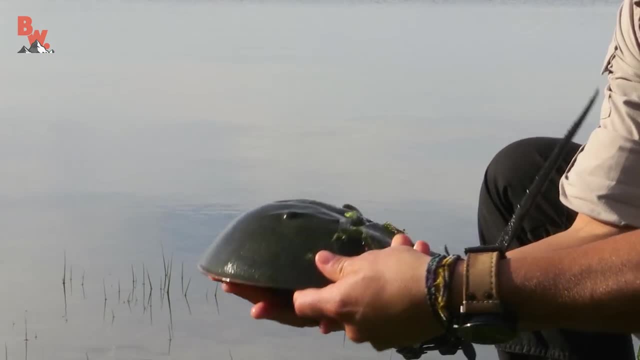 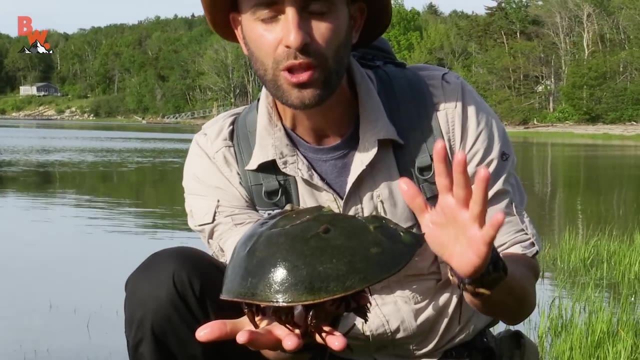 Let me see if I can get it to just lay in the palm of my hand. Oh, that feels really, really creepy. Now it's called a horseshoe crab, but it's not actually related to crabs at all. It's more closely related to spiders and scorpions. 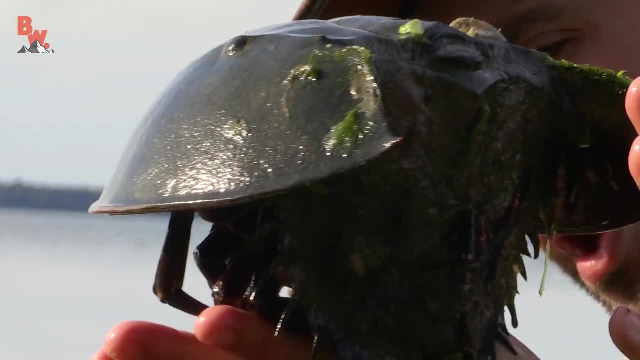 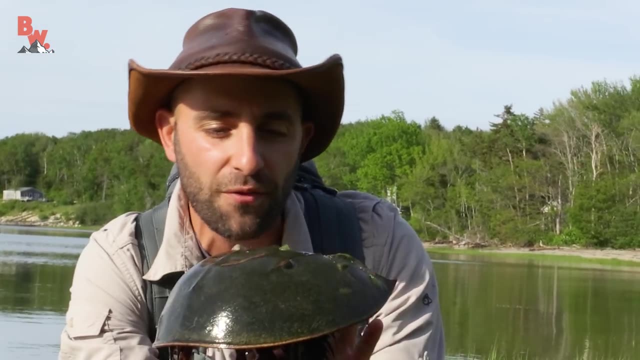 This is one large arthropod. Now wait, Oh, it is pinching me a little bit. They do have these front pedipalps up front that they use to harvest food off of the basin of the ocean. Wow, I'm like so excited right now. 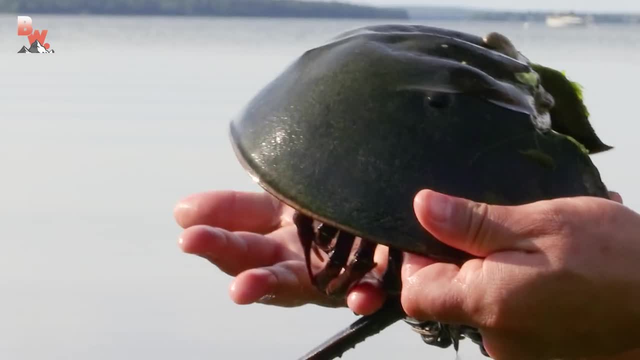 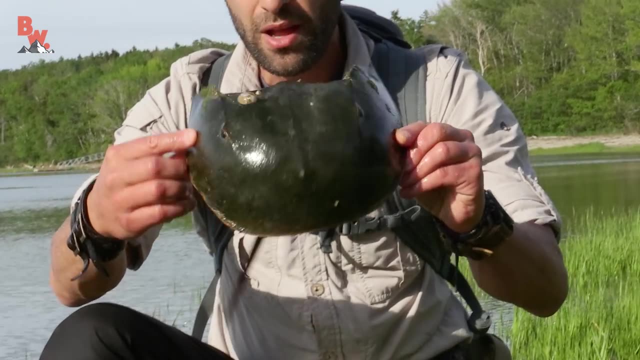 Hold on, I've got to compose myself because I did not think we were going to come across a horseshoe crab out here. Now, if you look straight on where it gets the name horseshoe crab, let me hold it like. 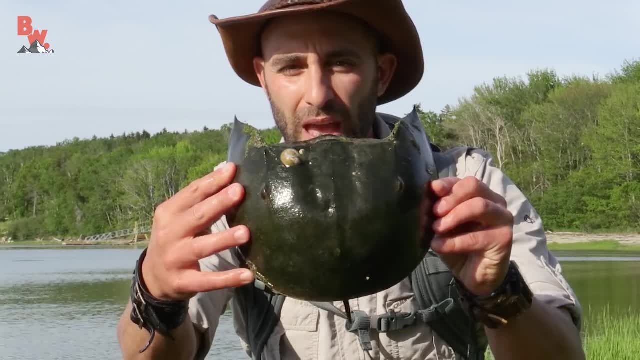 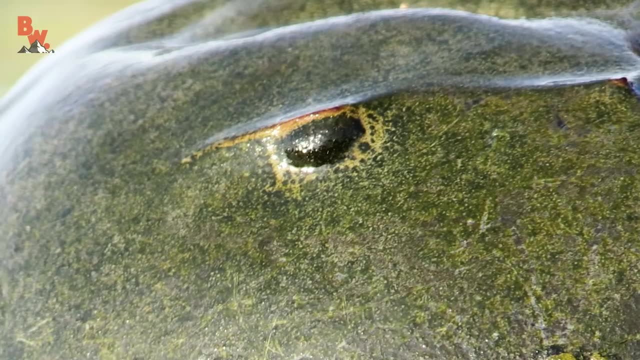 that looks just like a horseshoe right Totally. And if you look right at the front of the face there you see these little spots. Those are compound eyes. Actually, this animal has nine eyes in total- The two right here, five light sensing eyes on each of them. 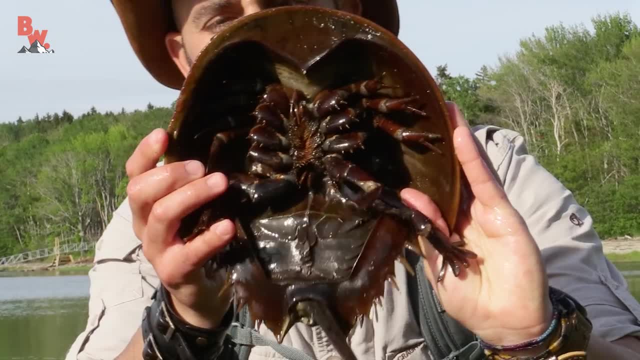 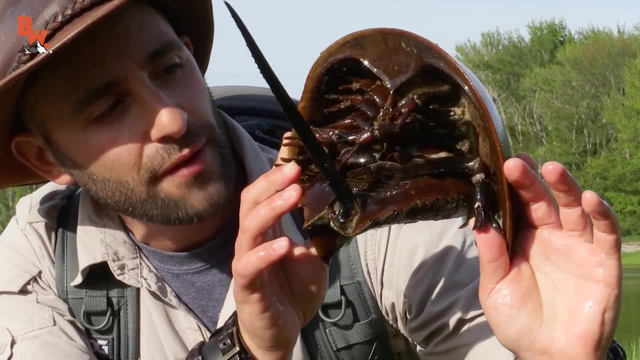 On top of its carapace and then on the underside, two simple eyes that they actually use to sense their environment. Scientists think that the eyes on the underside are actually just left over from when they were in a larva stage. Wait, Those are eyes on the top of that. 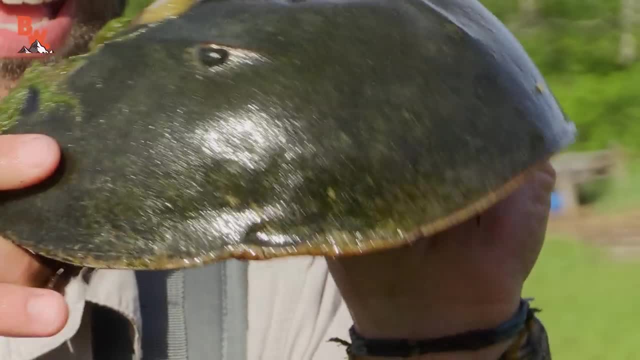 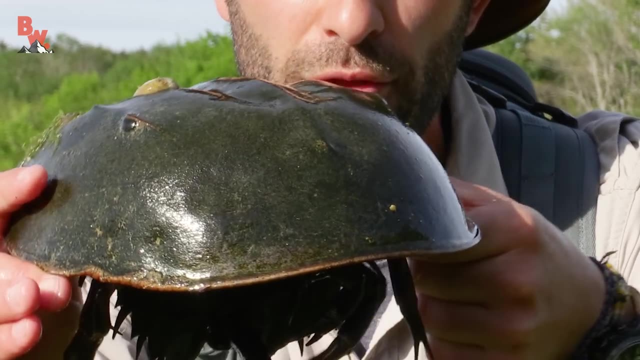 Yes, Actually it looks like a face, doesn't it? You see that I always thought that that was just like a helmet, like a shell protection. Well, the top of this animal is called the carapace. Just like a lot of other arthropod species, this is a very dense, very hard exoskeleton. 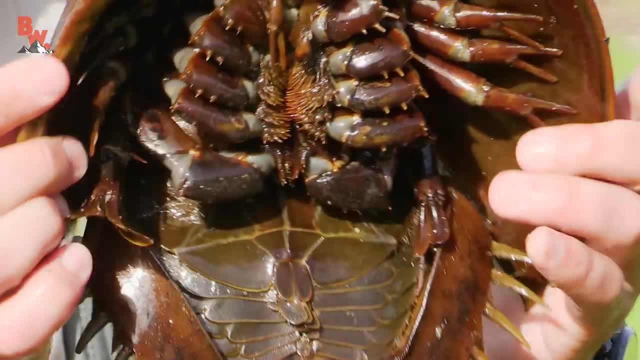 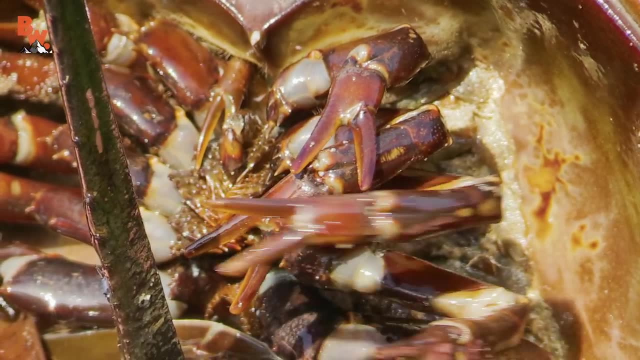 They don't actually have an endoskeleton. You know bones and cartilage like a human, But on the underside- look at that- It looks just like a scorpion or a spider. Whoa, Can I touch the top of it? 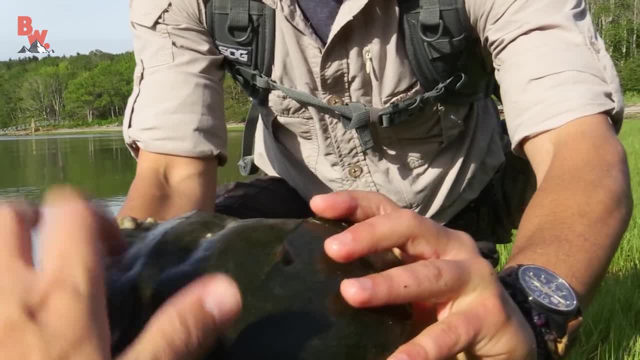 Yeah, yeah, yeah, Totally safe. Is it tough? Yep, Oh wow, Yep. Exoskeleton- It's just like a turtle shell actually. Yep. Well, I thought it was a turtle when we first walked up. 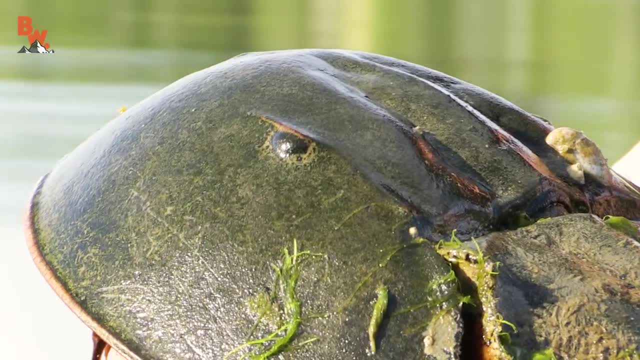 And look, you've got some sort of a barnacle growing up on top of it. It's covered in a little bit of algae and seaweed. Now here's something that you may not know, and something very cool. Let me turn it like this and just hold it in the palm of my hand. 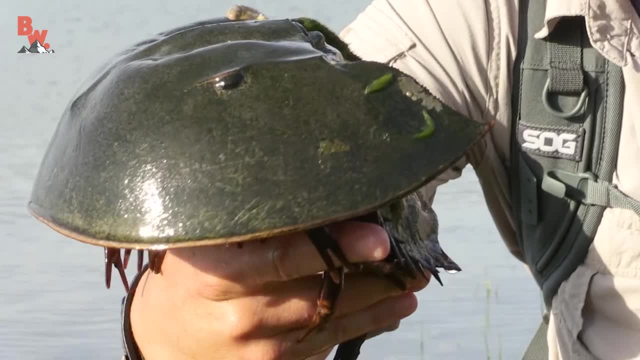 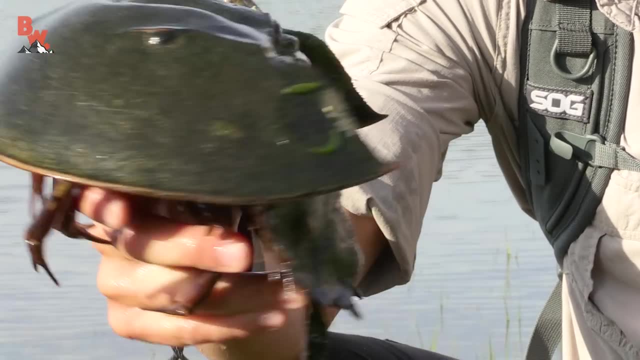 That is me holding a living fossil. The ancestors of the horseshoe crab have been on the planet for over 450 million years, And this species right here is the Atlantic horseshoe crab. There's only four horseshoe crab species in the world. 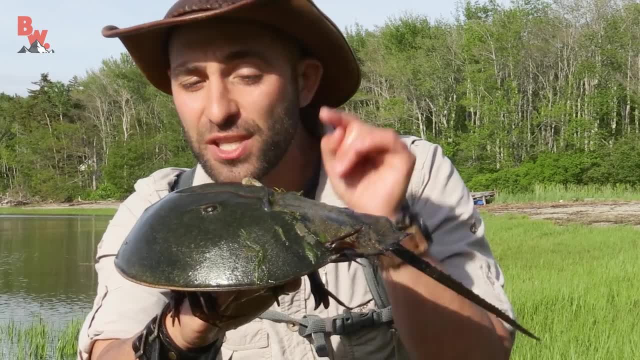 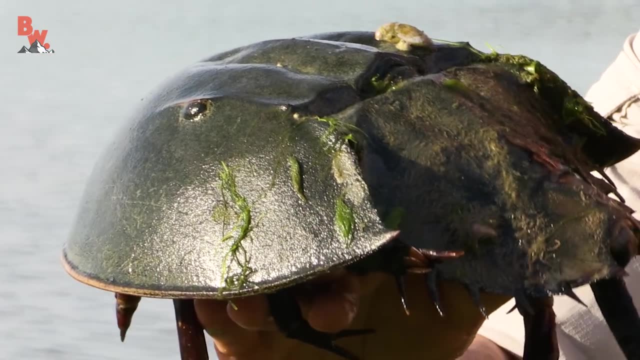 This is the only one that can be found off the coast of the United States, And this one specifically. this design- the Atlantic horseshoe crab- has not changed in over 230 million years That dates back to the Triassic period. 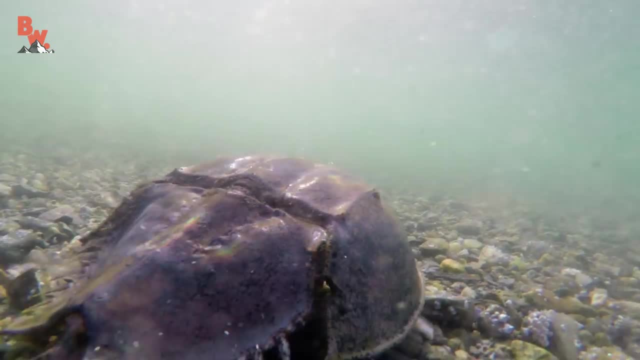 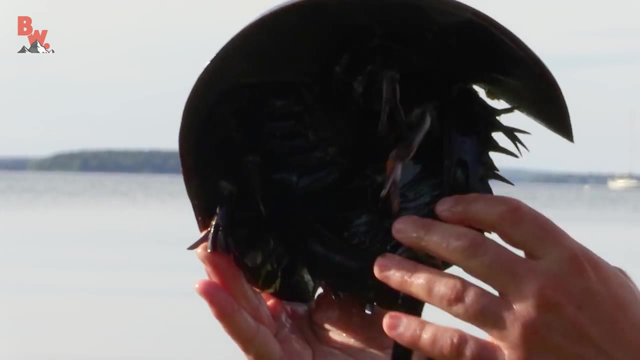 So this creature was crawling around on the basin of the ocean during the time of the dinosaurs. How cool is that Now they do get quite a bit bigger than this, And I'm guessing this is a female. The females are about 25% larger than the males. 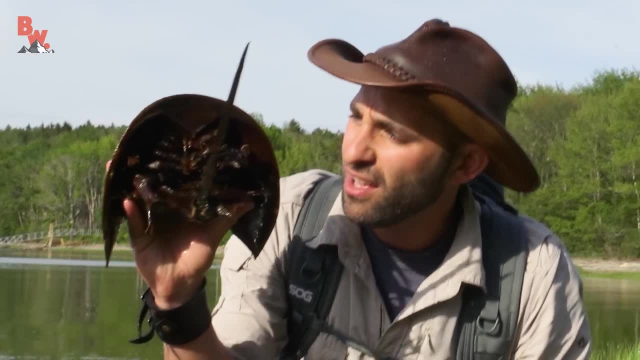 Wow, It's almost impossible to hold onto. Look at the underside. It does look like a stinger. It does, And that's why people are afraid of these things. They think that they're going to get stung. Look at this. 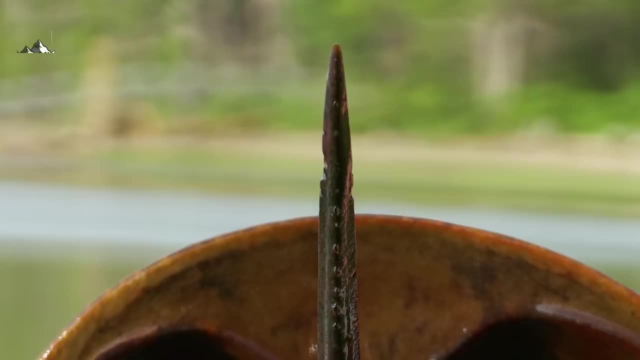 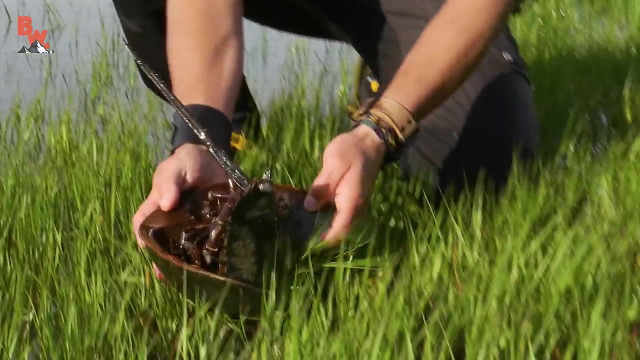 No, This tail is actually just used like a rudder, although it does have all these barbs. It's very intimidating, but it cannot hurt you at all. In fact, if a horseshoe crab gets flipped over, if a horseshoe crab gets flipped on its back like that, 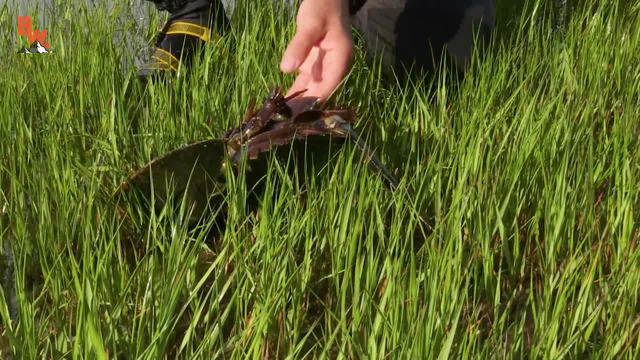 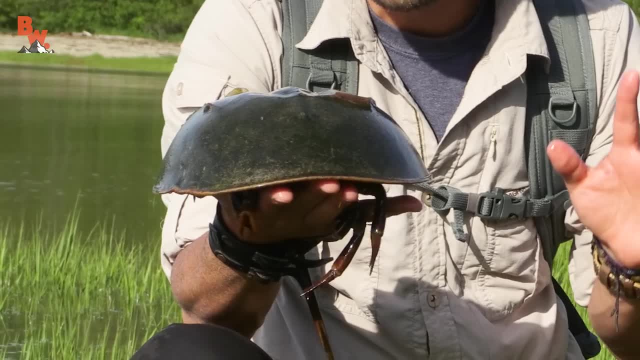 see it tries to right itself up. It actually can't, And that's a big misnomer that these arthropods are capable of flipping themselves back over, And there's actually a conservation effort that was launched in the 80s called Just Flip'Em. 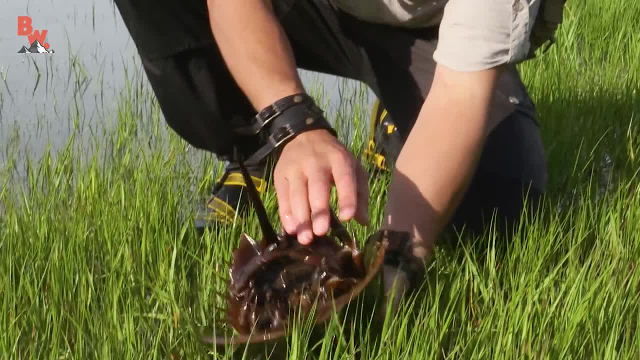 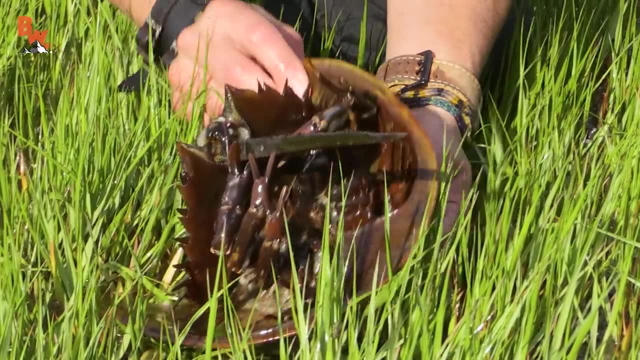 And the Just Flip'Em concept is that if you're walking down the beach and you see a horseshoe crab that's flipped on its back like this from like a crashing of a wave, what you're supposed to do is gently grab the carapace and flip it right side up. 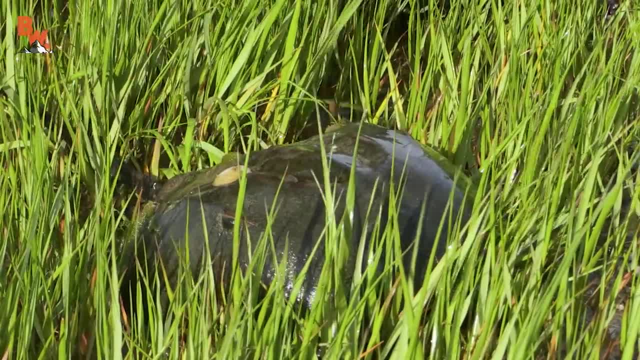 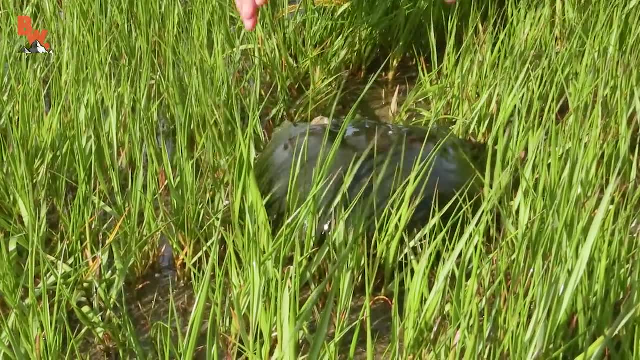 Now, you don't want to pick it up by its tail, because you can actually injure the animal if you hold it like that. Look at that, Mark, It's coming right towards you. Oh man, Do they ever come on land for anything, or are they purely aquatic? 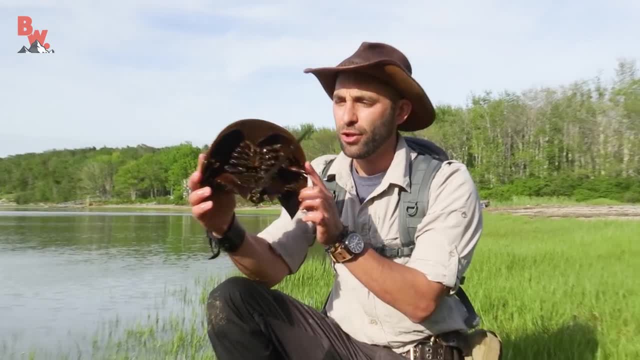 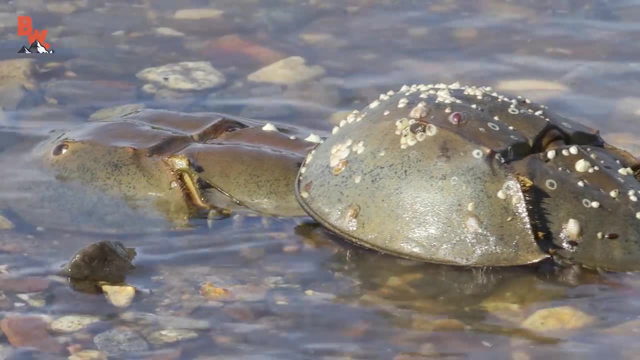 Well, between June and August they come very close to shore to breed, And the way that they do that is, the female will kind of nestle down in the rocks and a male will come in and latch himself onto the back of the female. 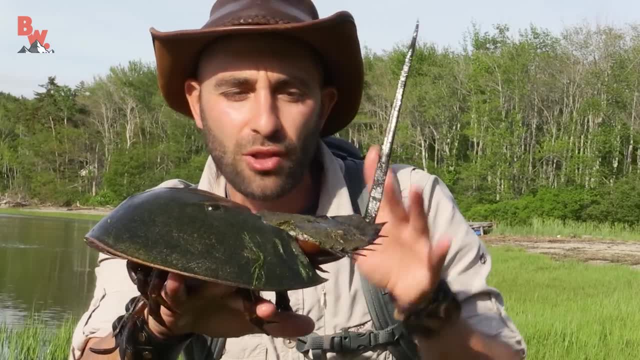 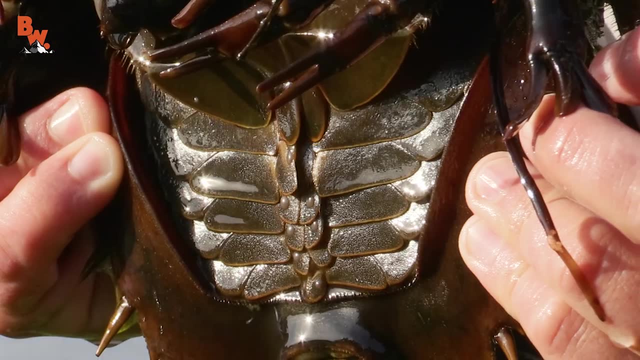 Horseshoe crabs can breathe underwater or out of the water Because a lot of the time when breeding is taking place, sometimes they're caught as the tide goes out too quickly and they can actually breathe air. Wow, I have really wanted to feature a horseshoe crab on Beyond the Tide. 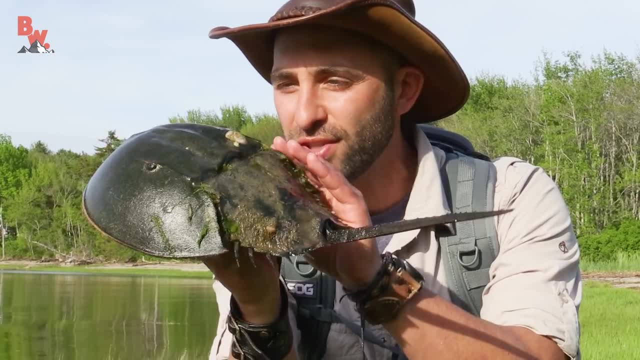 and it's kind of being in the right place at the right time that we came across one of these giants. Look at that thing That's as big as my face is. Whoa. I do have to watch out for that tail, though. 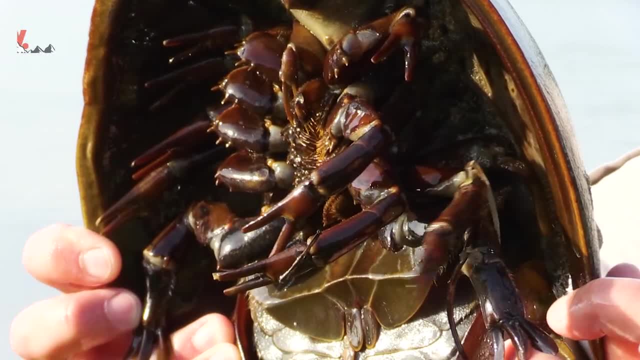 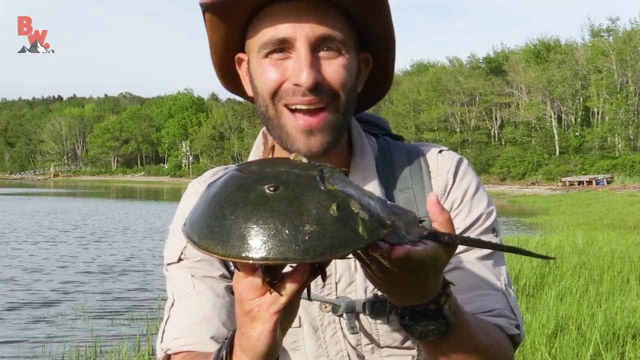 I don't want to get stabbed in the eye by it. Well, how cool was this? Coming across one of the most bizarre creatures you can ever see, One of the most bizarre creatures you can ever stumble upon in the tide pools: The horseshoe crab. 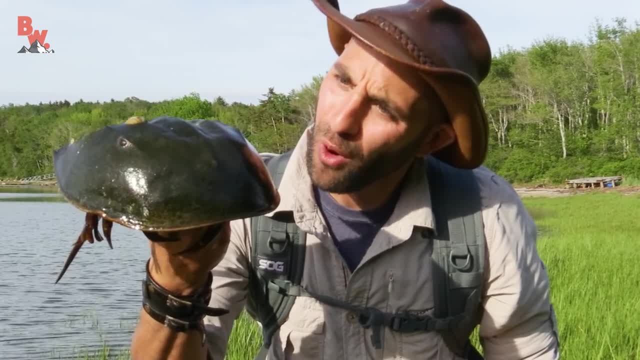 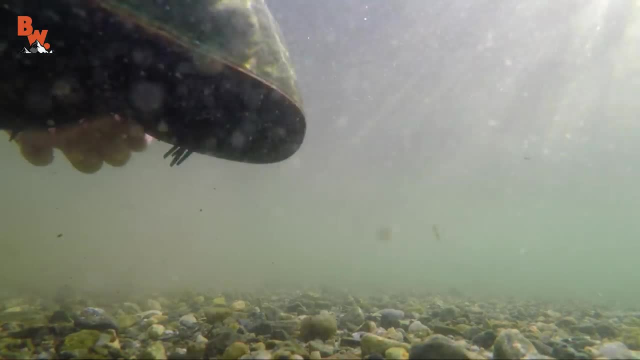 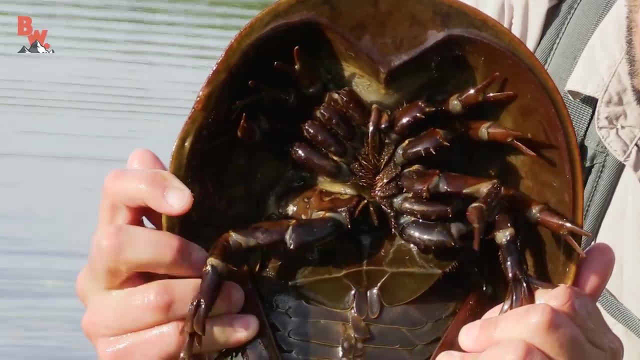 I'm Coyote Peterson. Be brave, Stay wild. We'll see you on the next adventure. All right, Let's let her back off into the ocean, Despite its angry appearance, intimidating spiked tail and creepy set of legs and pinchers. 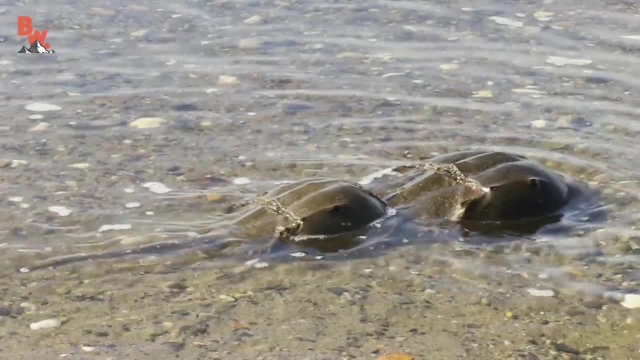 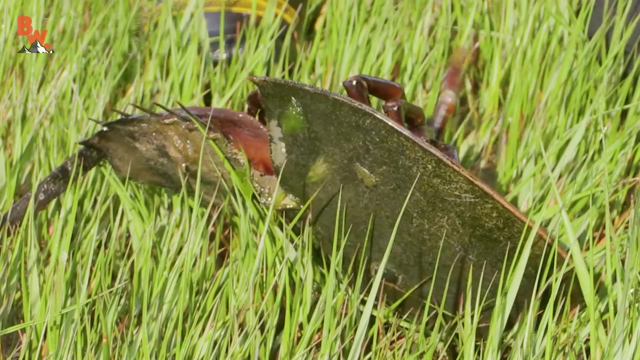 the horseshoe crab is one of the friendliest marine animals you can stumble upon. If you see one in the wild, simply admire it from a respectful distance. If you see one flipped on its back, have no fear when it comes to picking the animal up.